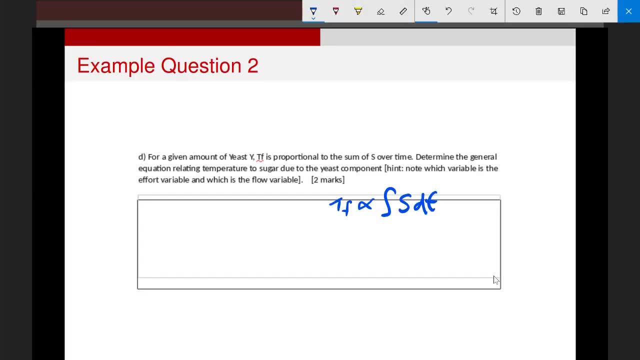 S over time. So that's an integral symbol and this dt means over time. This is a general relationship. To turn it into a general equation, we would have: TF equals K, integral S dt. What did I do? I put this K value in here. K is the constant of proportionality. 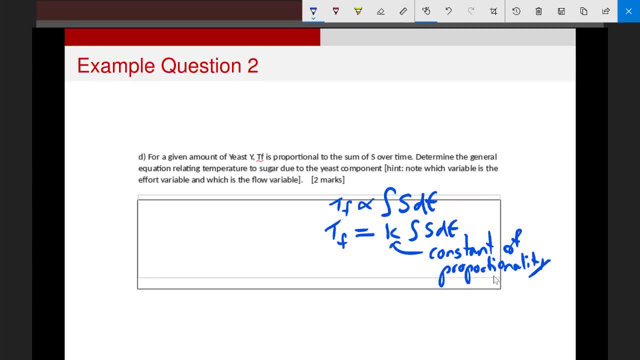 And yes, I don't have enough information in the question to know exactly what that is. I might make an educated guess because it says for a given amount of yeast. So I might say that the yeast content is the constant of proportionality. but I'd be better to say 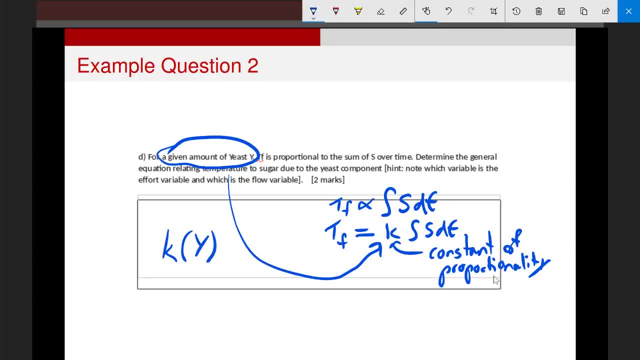 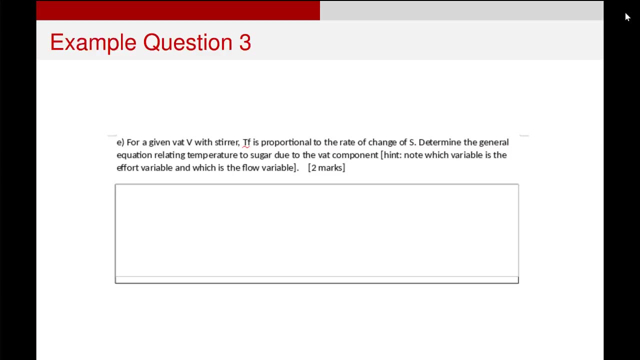 that the constant of proportionality is probably just a function of the amount of a given amount of yeast, rather than just saying it is Y specifically. Let's have a look at another question. The next question will be similar. The next question will be similar, but it has some different properties. So it says: 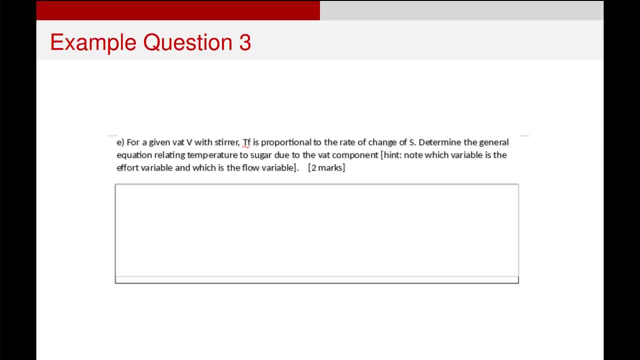 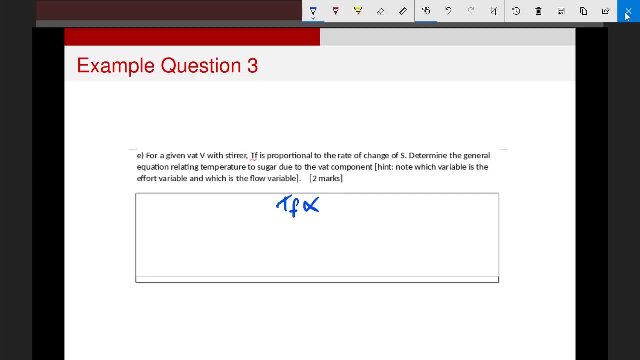 now for a given vat, the fermentation temperature is proportional to the rate of change of the amount of sugar. So how do we answer that? Well, exactly the same way. We'll start out with a general relationship saying that TF is proportional to dS over dt. Why? Because 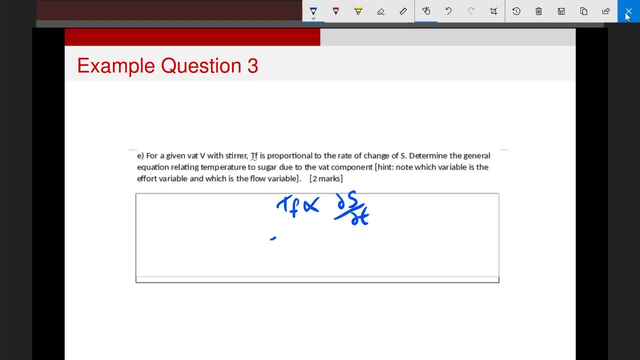 this is shorthand for the rate of change of the amount of sugar. We turn this from a general to a specific relationship by going K dS over dt. Once again, that is the constant of proportionality and once again I might say that that is just. 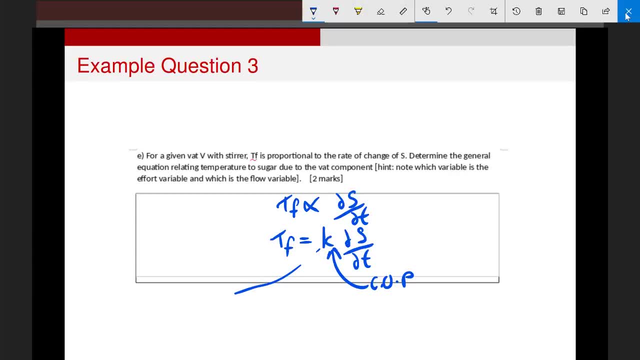 V, the given vat. but I would prefer it's more accurate to say that K is probably a function of V, because it's not clear to me from this question that the only important thing relating the rate of change of the sugar content to the fermentation temperature is. 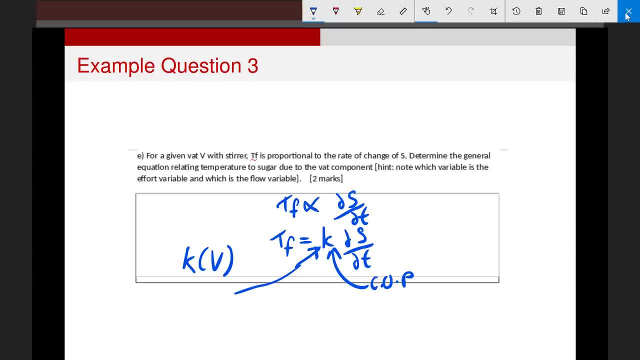 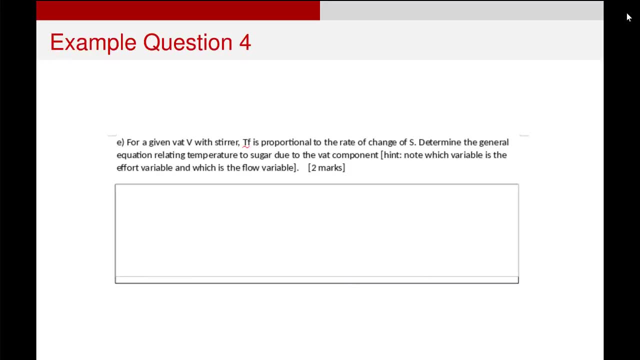 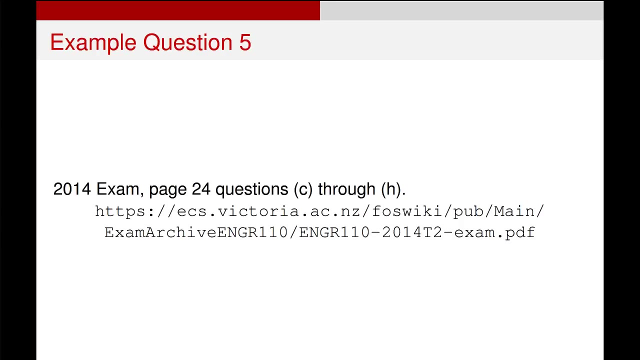 the size of the vat. There's probably going to be other things in there as well, So I prefer to use this general K term rather than a specific V. So there's lots of other equations you can find on. sorry, lots of other problems and examples you can find online to go through these kind of questions.